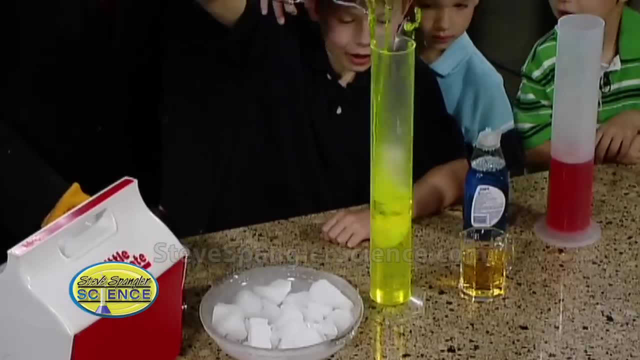 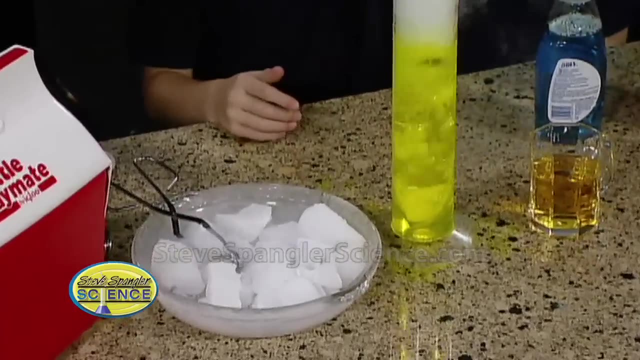 what he thinks about the water temperature. More screaming is always good. What do you think? What do you think So, hot or cold? What do you think, Mr Kovrig? Should it be hot or should it be cold? Hot Right, because it brings out that really. 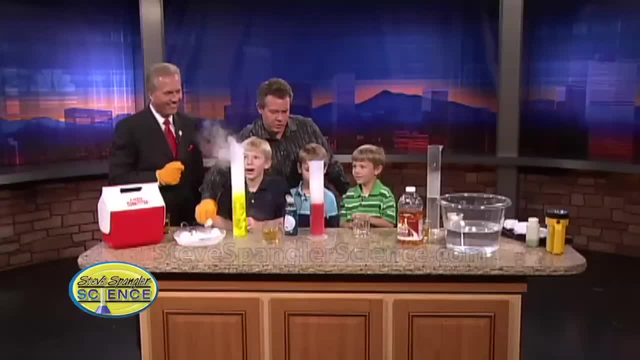 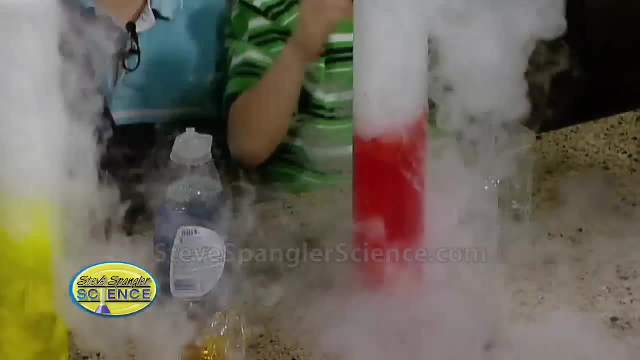 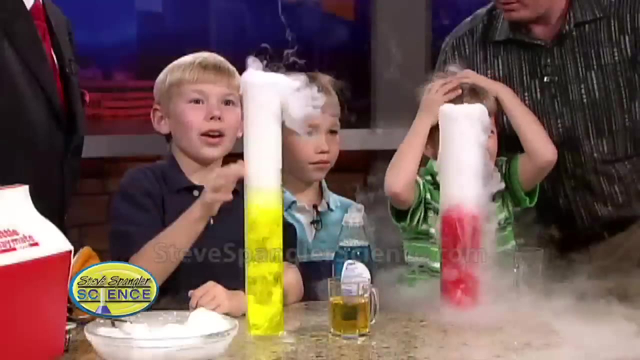 spooky effect. That's it. Oh, yes, it is A spooky effect. Good job, All right. So, Mark, while they're playing with that, would you tell us about yours? What do you think about yours? Well, we'll watch. If you really want to have some fun, then buy some soap pour it. 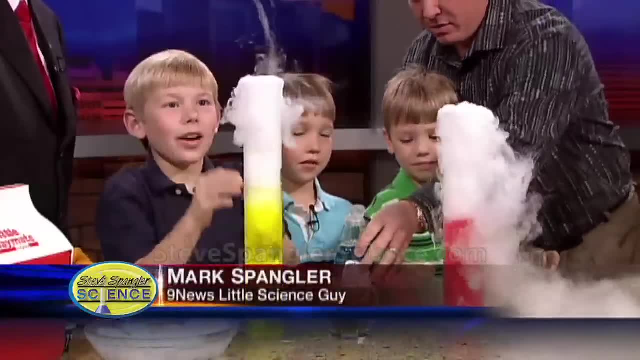 into the, Pour it into the soap. Yeah, So I'm going to pour it into the soap. Yes, So I'm going to pour it into the soap. And then you're going to put it in the cylinder Right And watch out. 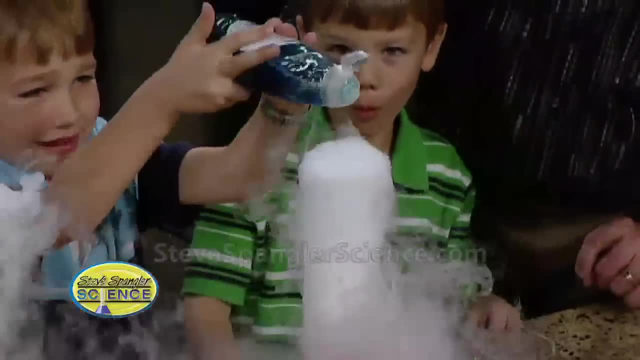 Okay, let's do it. Show everybody the soap. So the soap is going to go inside. So go ahead and put the soap in. It's okay. All the spending children know that phrase. watch out, Yes, Yes, There, you go A little bit, there is good. 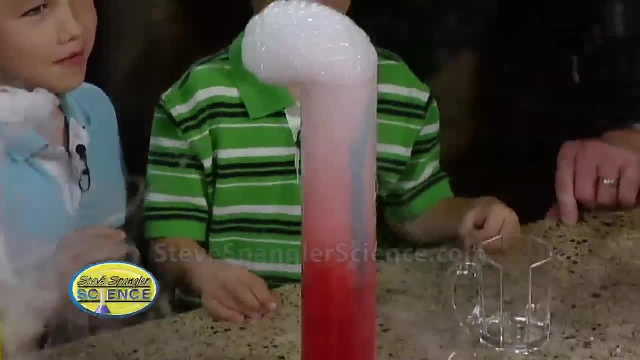 Yes, Three drops are good. Then half the bottle is Oh, Oh, Oh Wow. A little bit of you, I guess, Oh, Wow. So now this is pretty cool because the kids can touch it. Now I just can't get it to. 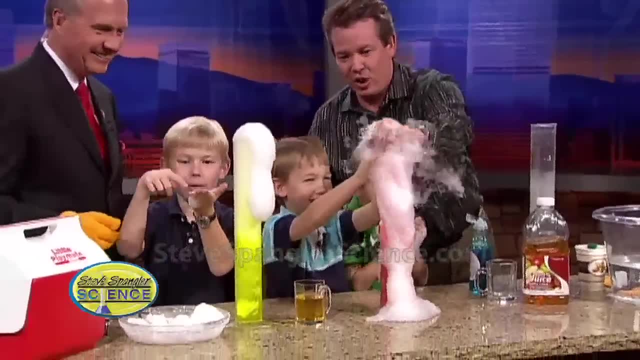 I just can't get it to stop. but it just keeps on going and going. Now it's filled with carbon dioxide, so it's safe, And we like these graduated cylinders because the kids can't get their hands down on the graduated cylinder. 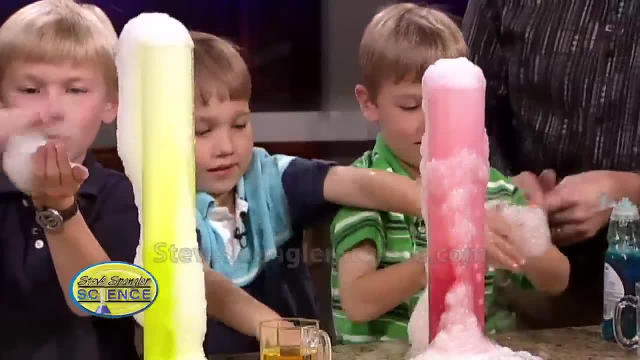 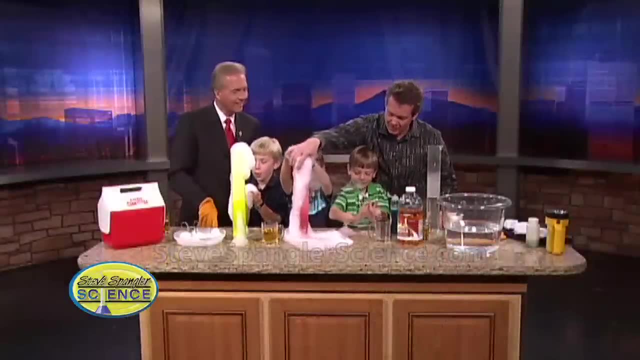 And this is what Halloween looks like the whole night. all right, All right. so, Scotty, pretend like you're not playing with that anymore and let's play with this. What is this? Well, you just need a little bit of apple juice and some dry ice. 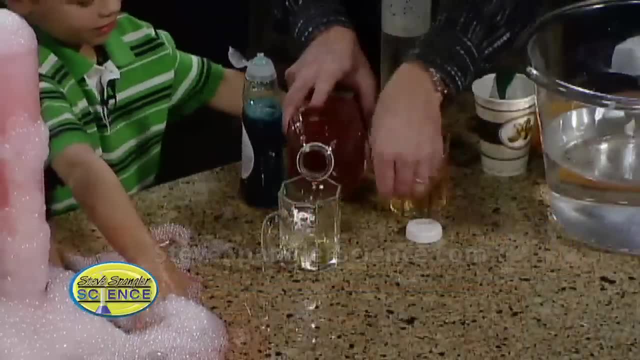 Oh, apple juice and dry ice. So we put a little bit of apple juice in here like this. so a little bit of apple juice. If my hands weren't nice and wet, that would be great. And then we get a little bit of dry ice. 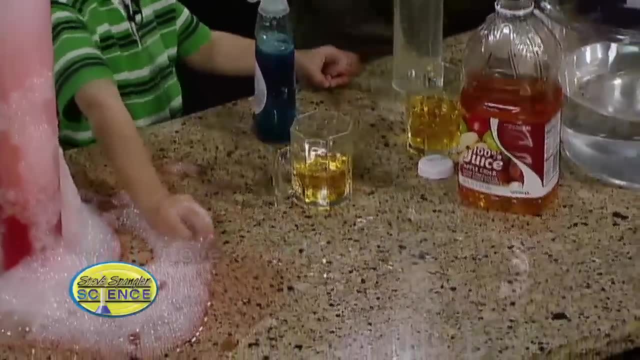 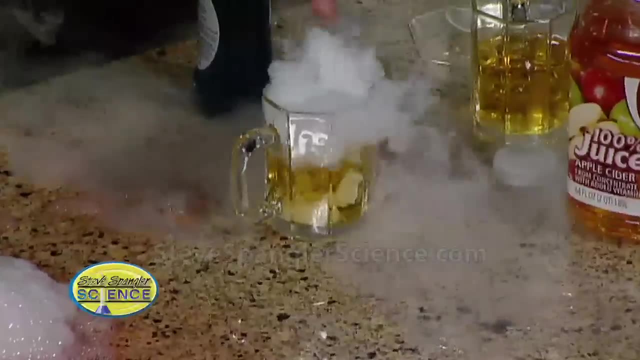 And now, what's the dry ice going to do to the apple juice, Scotty? Oh, it's going to make it bubble. see, Oh, bubble, bubble. toil and trouble. Have you seen that before? And we never serve it with the bubbling going on here. so we wait. 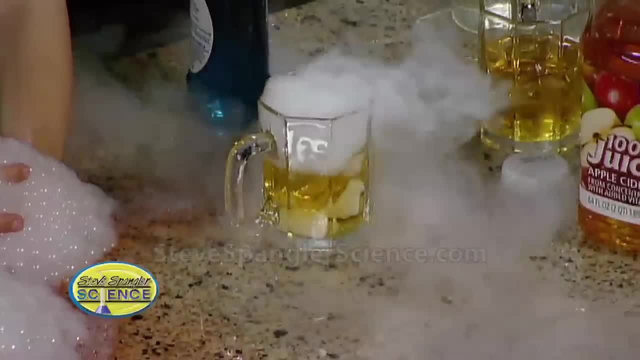 So, Mr Coburg, off to the side there, take a look at yours. Oh, you see this one here. So we don't serve it that way, but we wait until all the ice is gone and then we get a little bubbling drink.